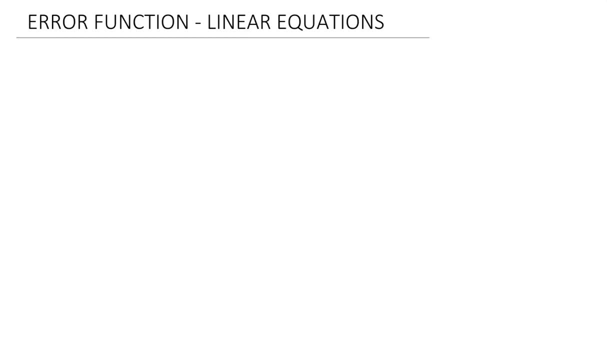 Hey guys, back with another video. In this one we will learn how to use the error function to evaluate some linear equations. and to start off, I will define the error function. We use three letters to denote it. It is erf error function of x and this is equal to 2 over. 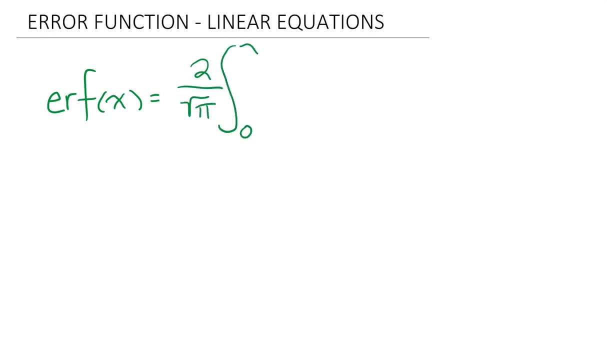 the square root of pi, times the integral from 0 to x of e to the minus t squared dt. Now it's important that we realize that this is a function of x and not of t. So I will draw the function e to the minus t squared here, and this is with respect to t on the x-axis. It looks sort. 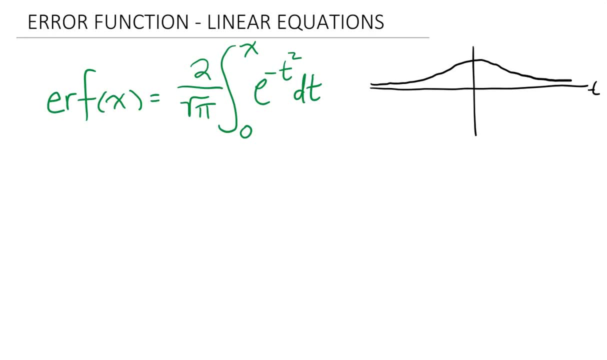 of like a bell curve and we will choose- well, we know this is 0, and we will choose some value of x and we will evaluate the integral underneath, or rather the area underneath this curve, from 0 to whatever value. We choose x, and that is what the error function is evaluating and, of course, it is taking this: 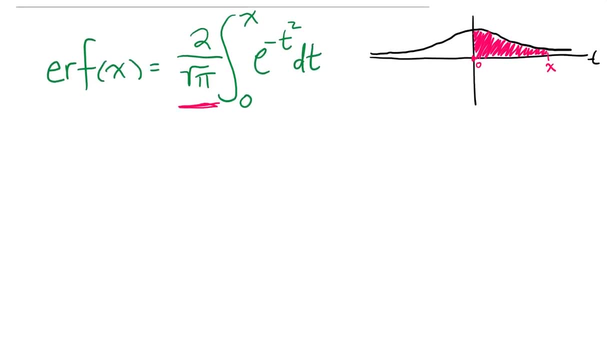 area, and it is multiplying it by 2 over the square root of pi. Now let's look at an example of a differential equation. So we have, for our first example, dy dx is equal to 2xy plus 1.. And so I am going to assume that you already know how to solve a linear equation that 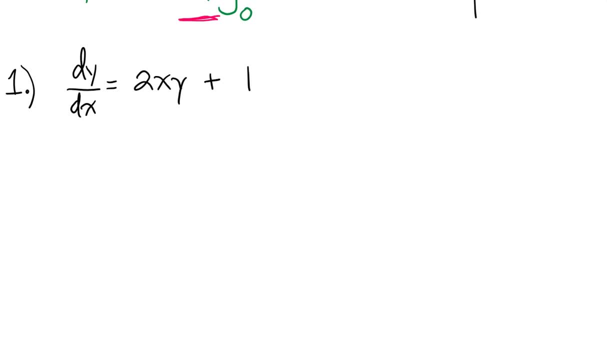 you have watched my last video. If you haven't, go give that video a quick watch and then you will be more prepared for the technique that I will do right now. So we will move the 2xy to the left-hand side. We get dy dx. 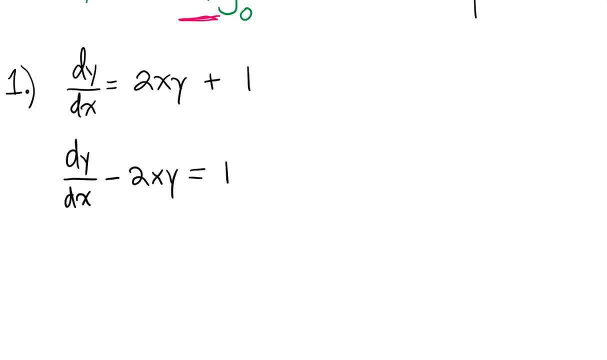 minus 2xy is equal to 1.. Now we know that our p of x is equal to minus 2x, And if we take the integral of minus 2x dx, what we get is minus x squared dx, minus 2x dx, minus 2x dx, minus 2x dx. 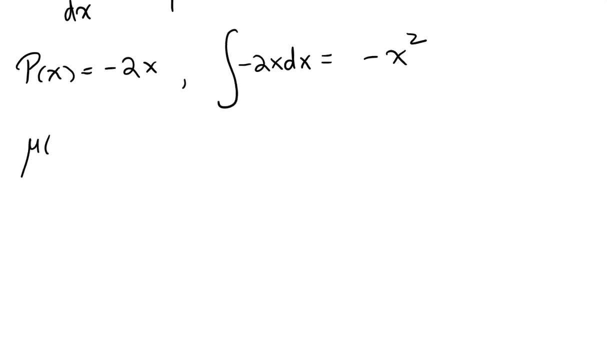 Now our integrating factor mu of x will equal e to the minus x squared. And if we multiply e to the minus x squared, our integrating factor so e to the minus x squared times y, and we take the derivative of this and we know that this will equal e to the minus x. 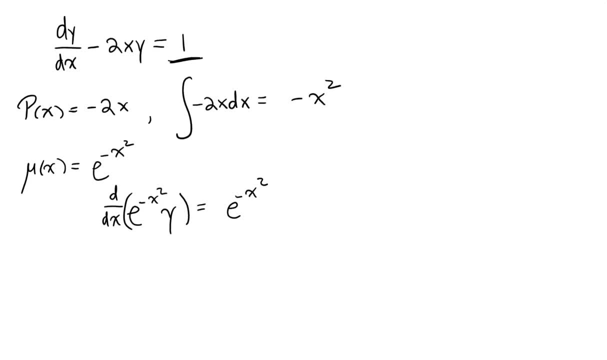 squared times our right-hand side, which is just 1.. Now let us, let us take the integral of both sides. so we will take the integral and normally, when we take an integral, we will take the indefinite integral, but in this case, what we will? 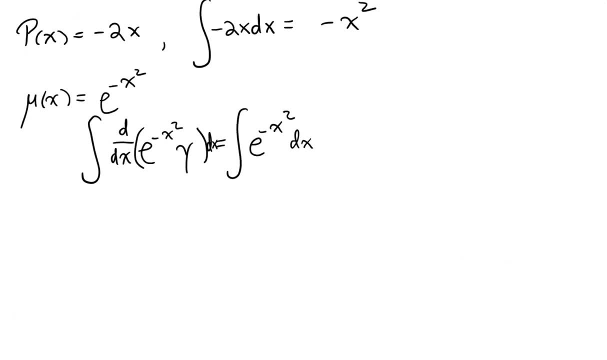 do is we will realize that on the right hand side we have the integral of e to the minus x squared DX, and this is not an integral that we can readily evaluate, because it is not an elementary function. so what we will do instead is we will define some of our bounds. we will say, okay, well, let's rewrite this. we will 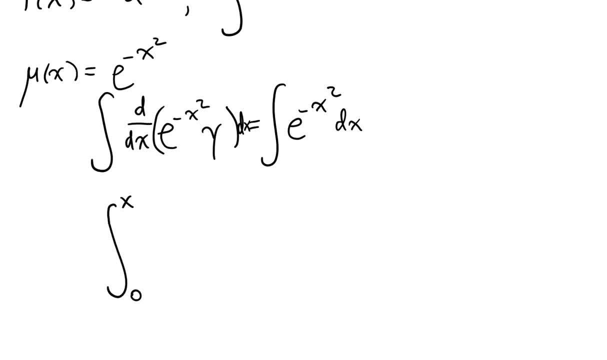 take the integral from 0 to X of both sides, so we get D, and now we can't do D DX, we have to choose some other variable, and as long as we're consistent we'll be fine. so that's D DX of e to the minus T, squared times Y, and remember that Y here. 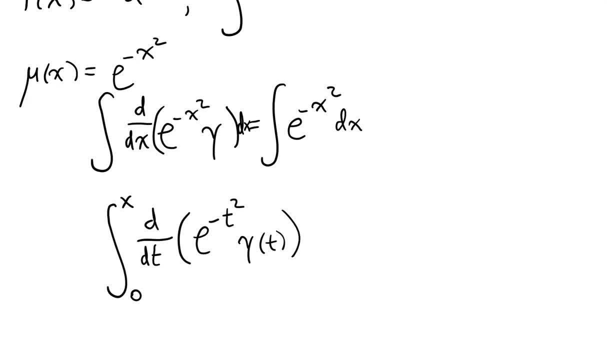 is a function of T. I'll just write it so we don't forget. and this is with respect to T, and we will take the integral similarly, on the right hand side of 0 to X, of e to the minus T squared DT. now I did forget to write one thing: this differential. 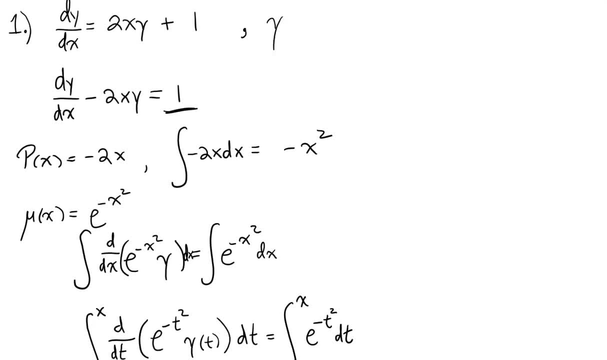 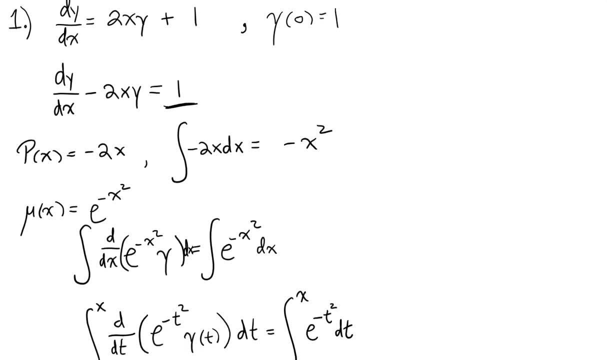 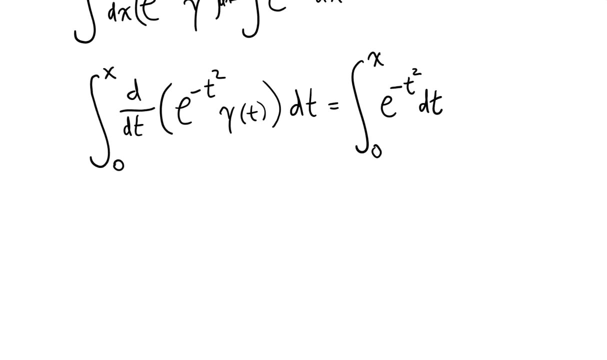 equation, we do have an initial condition, which is going to be Y of 0 equals 1, and it's an initial value problem and we need that initial condition to be satisfied. so but we do want to keep in mind it happens by the determinant equation and 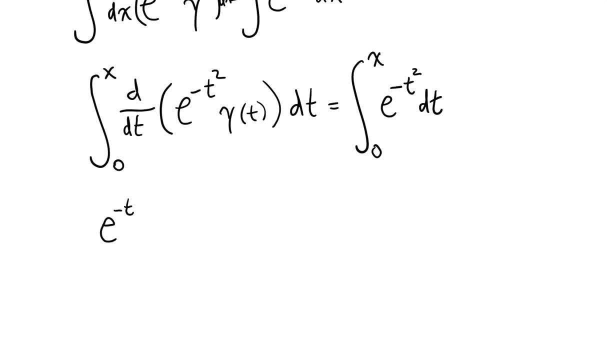 we combine it so we have the function of Y at the end of that team and we have our delta U and the delta Ahhh whenument vector and we change that data to the negative identity, and that was about 2 over square root of Y. and then now when 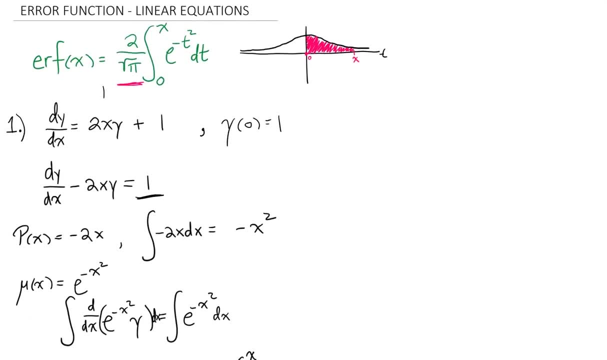 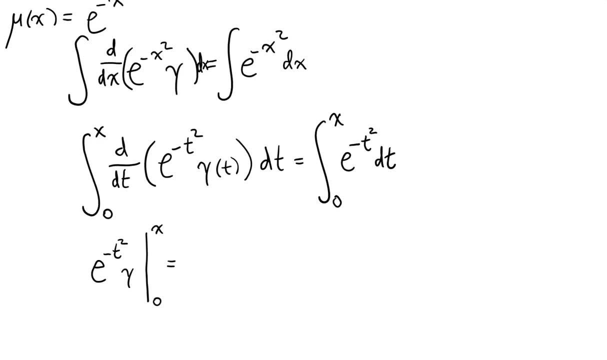 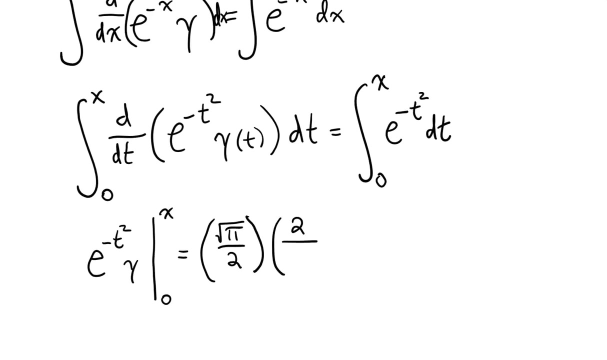 we evaluate the integral is well, the, the DD, T in the DT will cancel out and we. so what we can do is we can say: well, if that has the 2 over the square root of pi being multiplied by it, we can actually just multiply by the square root of pi over 2 and then multiply by 2 over the. 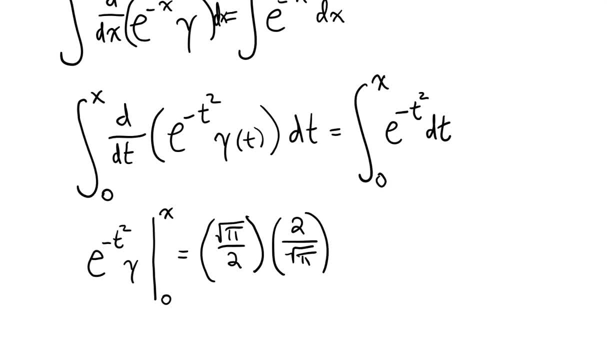 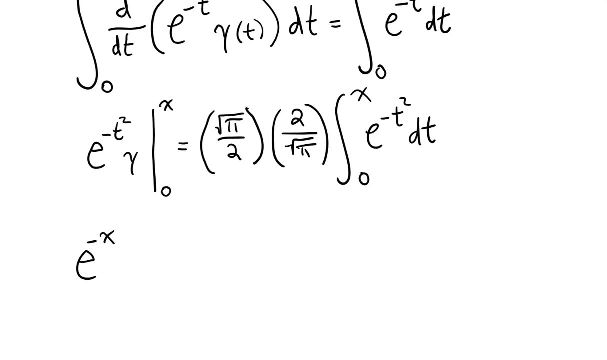 square root of pi, and these two cancel out to be 1, and then we can multiply this by the integral from 0 to x, of e to the minus t squared dt. if we plug in our bounds of integration on the left hand side, then what we get is we get e to the minus x squared times. y and y is just a function. 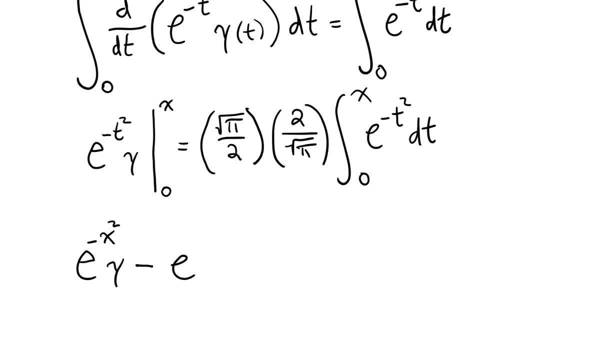 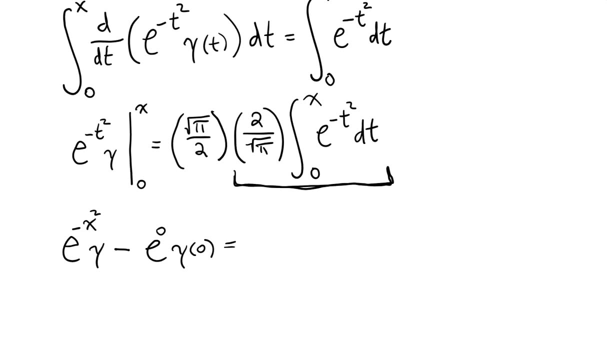 of x, and this will be minus e to the minus 0 squared, which will be 0 times y of 0, and this will be equal to. well, we have already defined the right side of of the right hand equation as the error function of x. that is what we defined in the beginning of. 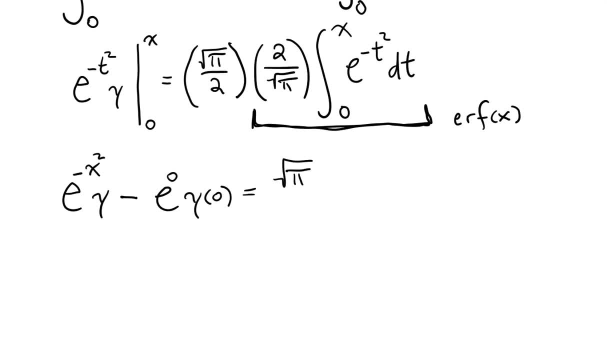 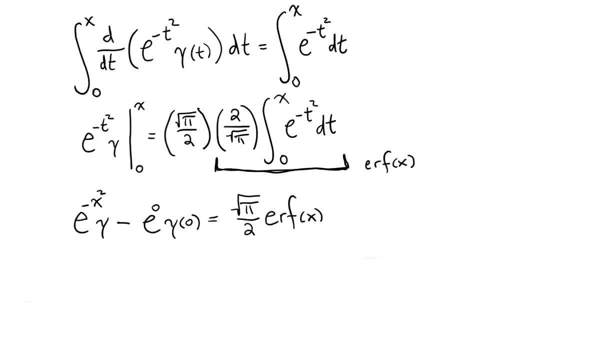 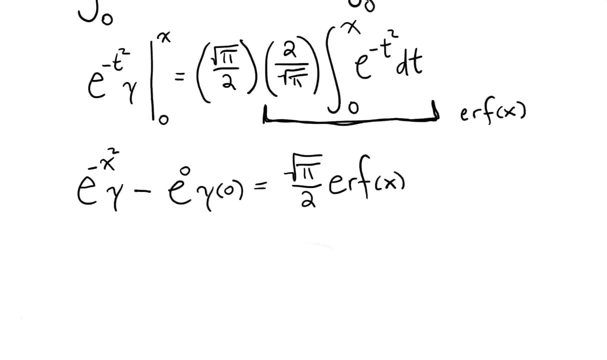 the video. So this will equal the square root of pi over 2 times the error function of x. and to satisfy our initial condition, we know that y of 0 is equal to 1 and e to the 0 is also equal to 1, so this will. 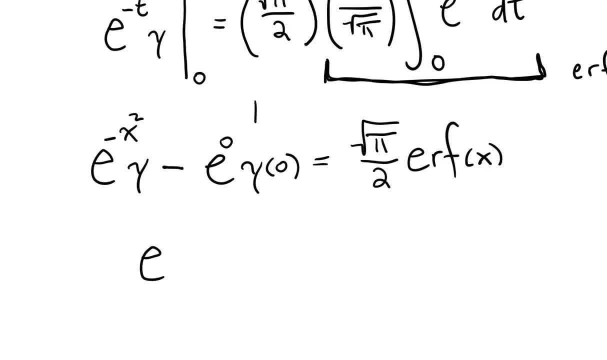 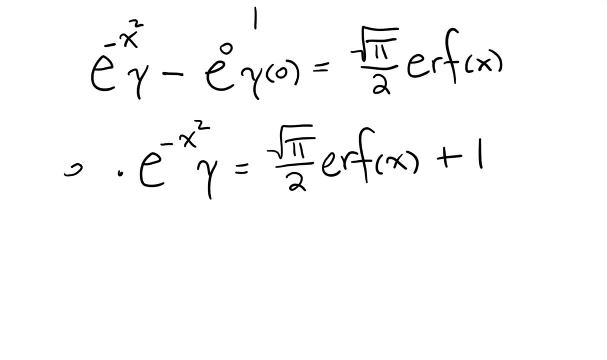 equal 1, and if we add that over then we get e to the minus x squared times. y is equal to root pi over 2 times the error function of x plus 1. now, multiplying both sides by e to the positive x squared, it will cancel out the e to the minus x squared on the left hand side. and then what we? 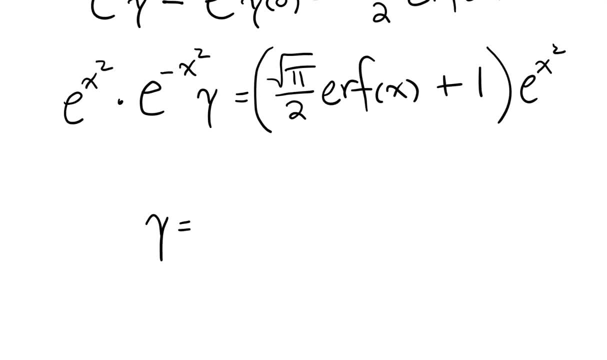 are left with as the solution to our initial value problem. note there are no plus C's or constants of integration because we have already solved for our our initial condition. We have e to the x squared times root, pi over 2 times the error function of x plus 1 and 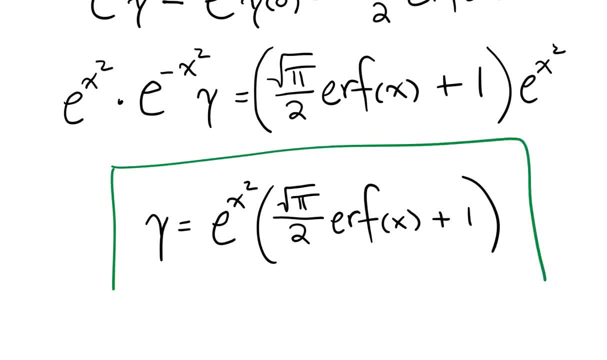 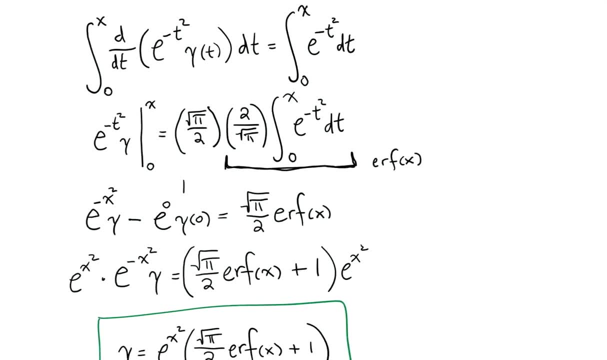 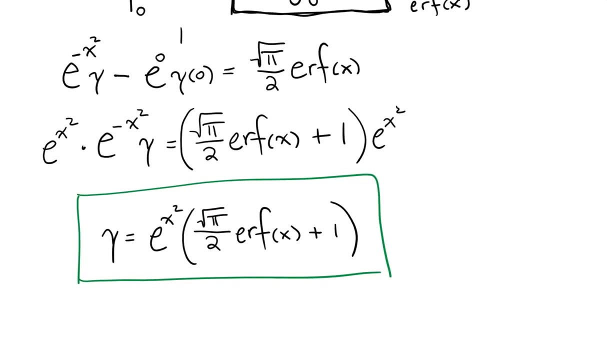 this is the solution to our differential equation. now the error function of x is very. it's a very succinct way of writing the large integral. it makes it a lot easier and a lot more neat for us to write. in the next video I will have another example.